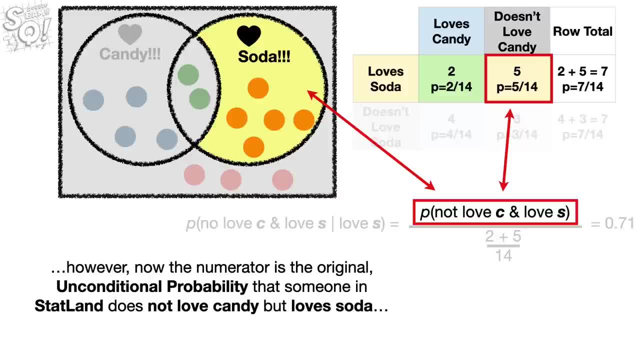 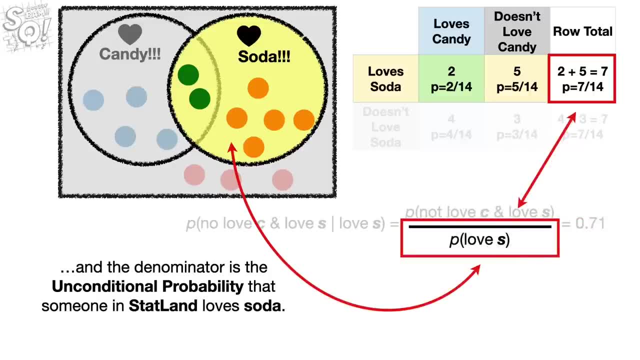 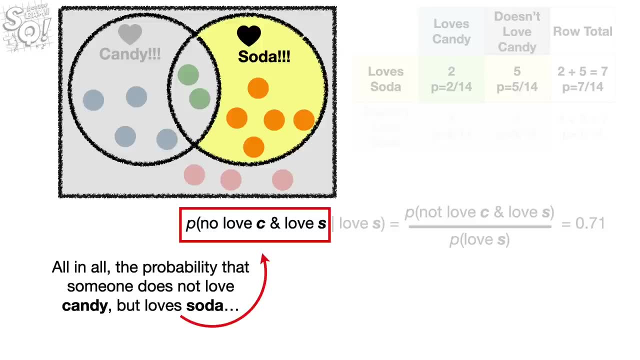 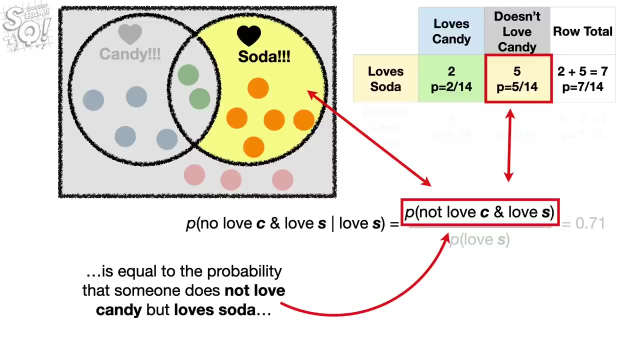 probability that someone in StatLand does not love candy but loves soda. And the denominator is the unconditional probability that someone in StatLand loves soda. All in all, the probability that someone does not love candy but loves soda is equal to- Given that we know that they love soda is equal to the probability that someone does not love candy but loves soda. 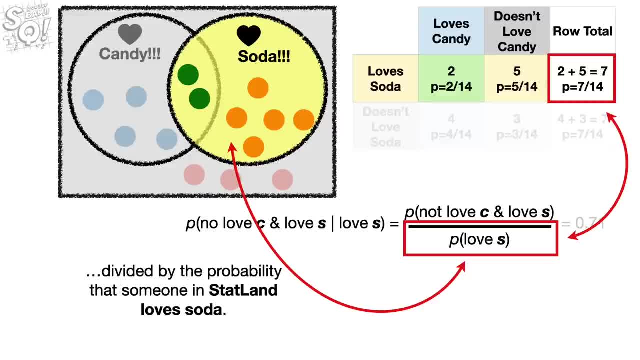 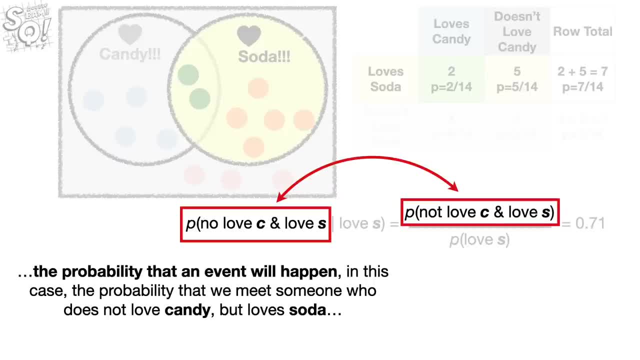 divided by the probability that someone in StatLand loves soda. So one way to think about conditional probability is the probability that an event will happen, in this case the probability that we meet someone who does not love candy but loves soda, scaled by the knowledge we already have about the event. 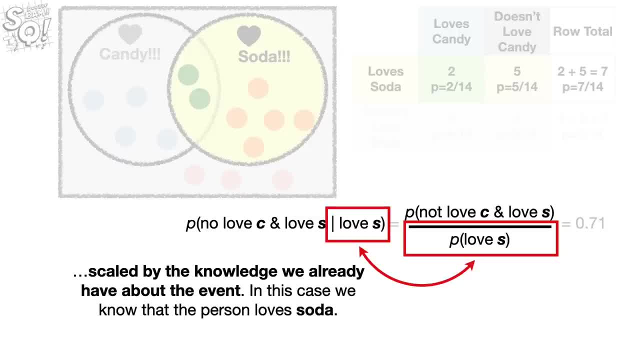 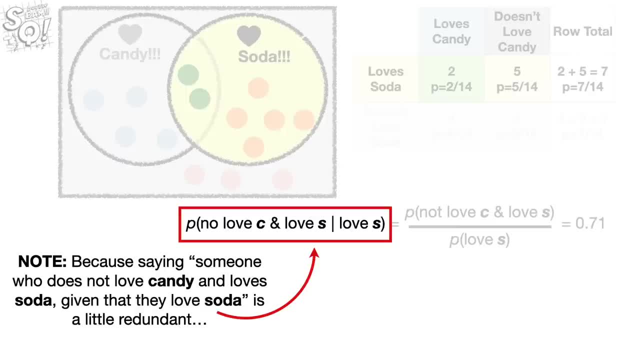 In this case, we know that the person loves soda. Note because saying someone who does not love candy and loves soda given that they love soda is a little redundant. many people omit writing out the and loves soda part and shorten the conditional probability statement to someone who does not love candy, given that they love soda. 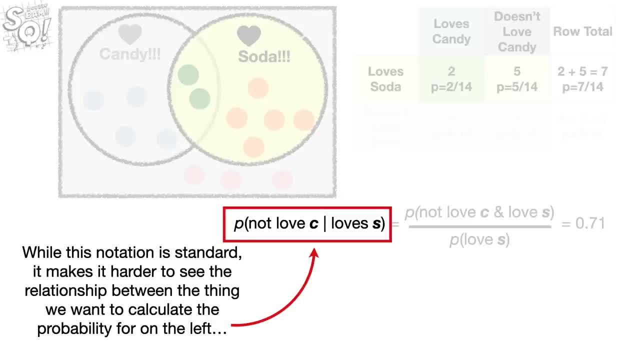 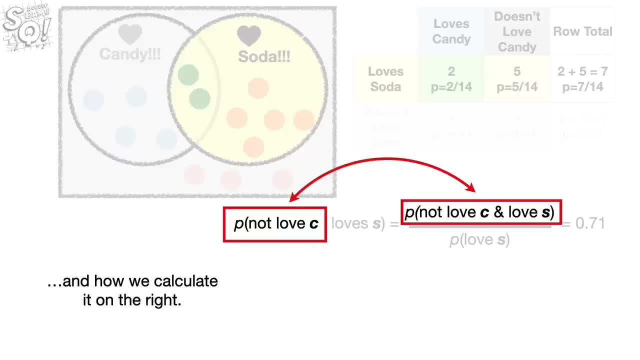 While this notation is standard, it makes it harder to see the relationship between the thing we want to calculate the probability for on the left and how we calculate it on the right. Using the slightly redundant notation for conditional probability makes it obvious that we want the probability that an event happens. 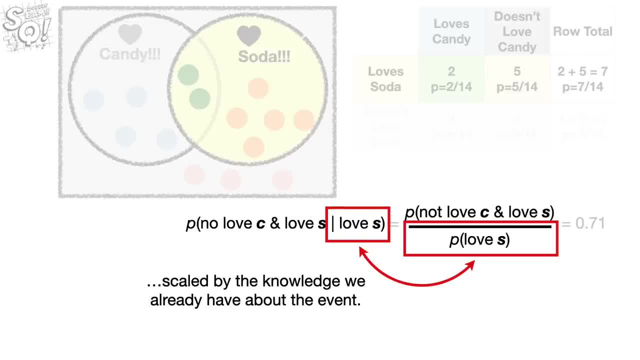 scaled by the knowledge we already have about the event. Personally, this slightly redundant notation is ideal, But there are only so many options that we can use in the case where an event happens, So we hurt the thought that we cal it because we don't know. 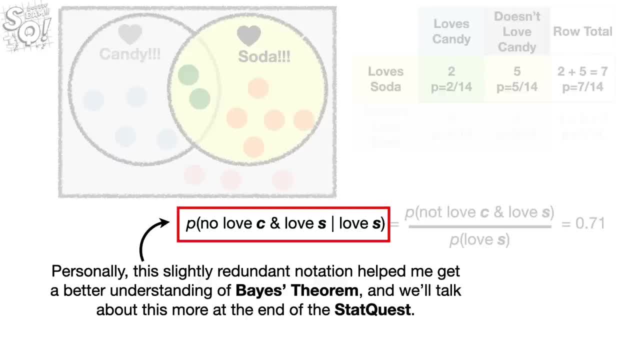 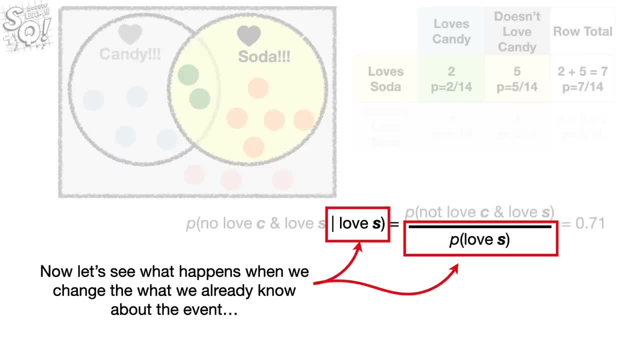 So we hurt the thought that we don't know. So we hurt the thought that we don't know helped me get a better understanding of Bayes' theorem, and we'll talk about this more at the end of the stat quest. Now let's see what happens when we change what we already know about the 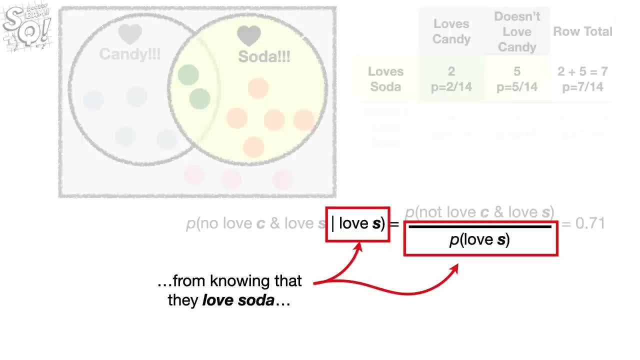 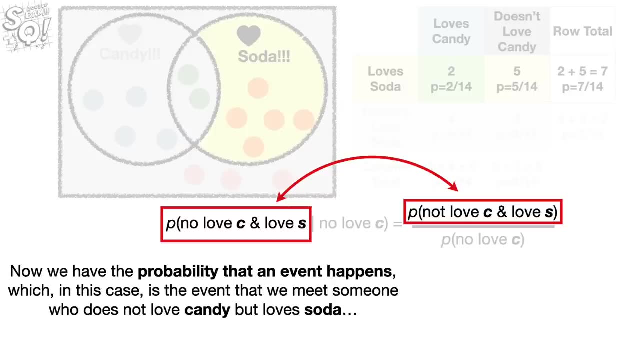 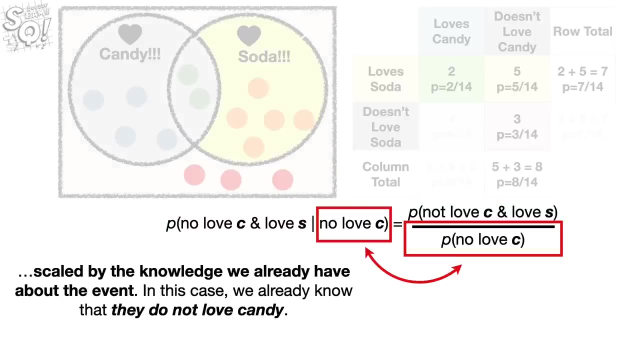 event, from knowing that they love soda to knowing that they do not love candy. Now we have the probability that an event happens, which, in this case, is the event that we meet someone who does not love candy but loves soda, scaled by the knowledge we already have about the event In this. 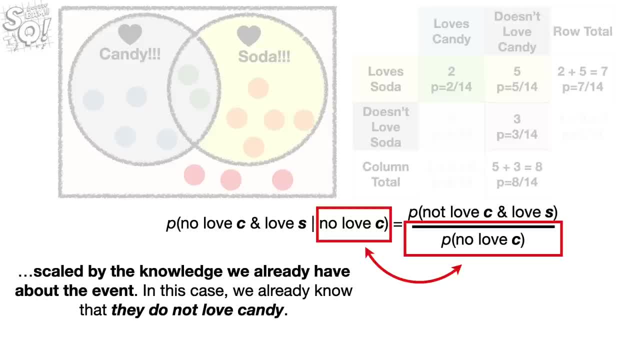 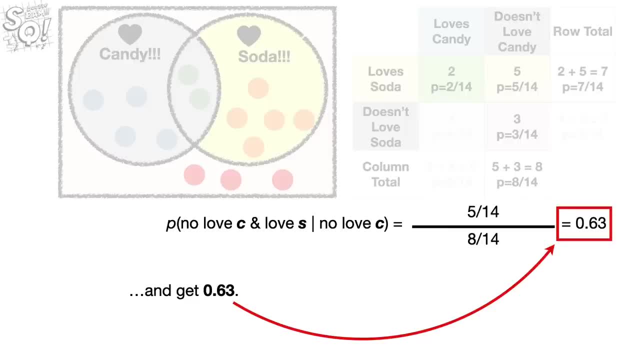 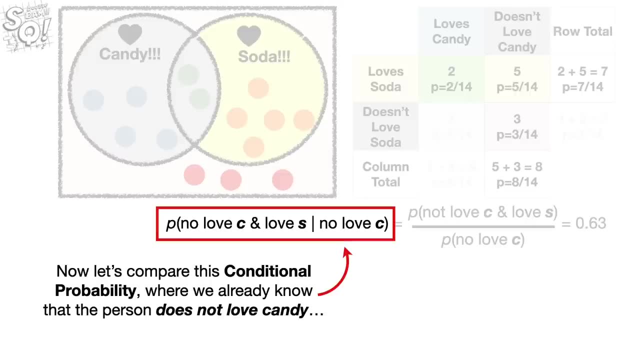 case, we already know that they do not love candy. Now we plug in the numbers and do the math and get 0.63.. Now let's compare this conditional probability, where we already know that the person does not love candy, to the conditional probability we calculated before, where we already 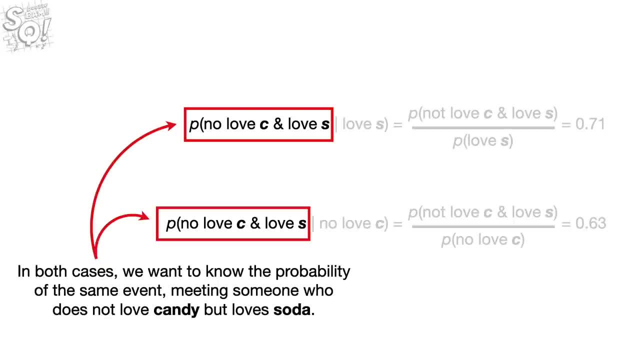 know that the person does not love candy. Now let's compare this conditional probability where we knew that the person loves soda. In both cases, we want to know the probability of the same event, meeting someone who does not love candy but loves soda, And that means in both cases. 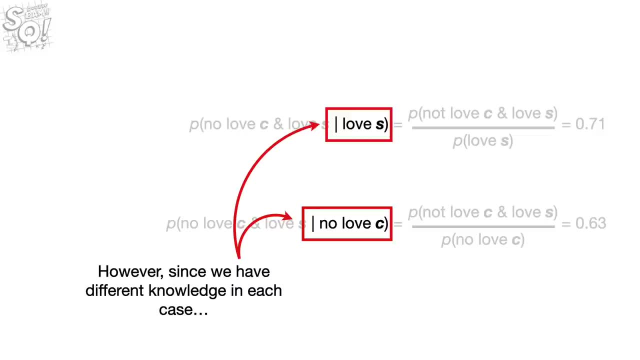 the numerators are the same. However, since we have different knowledge in each case, we scale the probabilities of the events differently And ultimately we get different probabilities. Hey look, it's Statsquatch. Statsquatch is our friend in Statland and he always wants to make a bet. 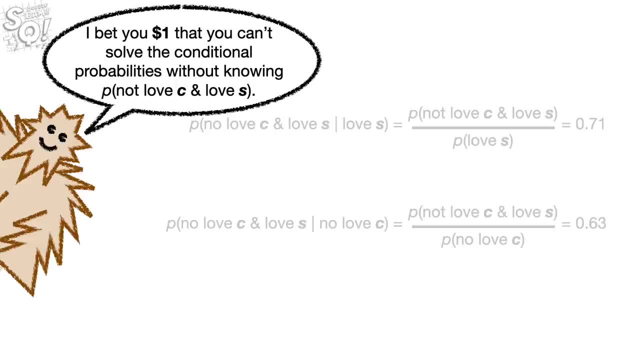 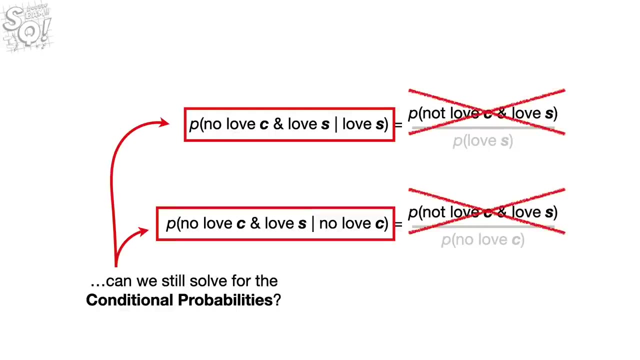 I bet you $1 that you can't solve the conditional probabilities without knowing the probability of not loving candy and loving soda. In other words, if we don't know the value for the numerators, can we still solve for the conditional probabilities? Well, even if we don't, 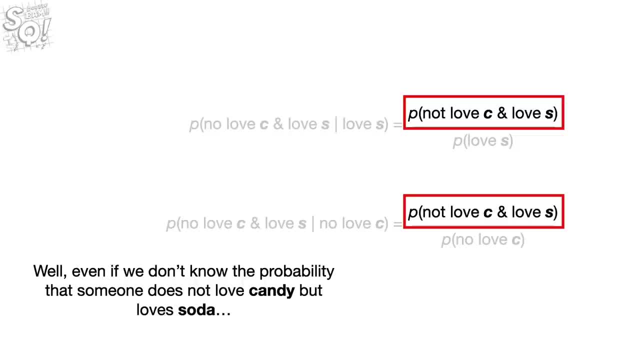 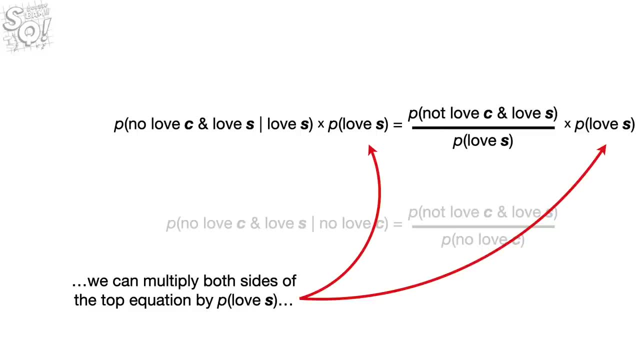 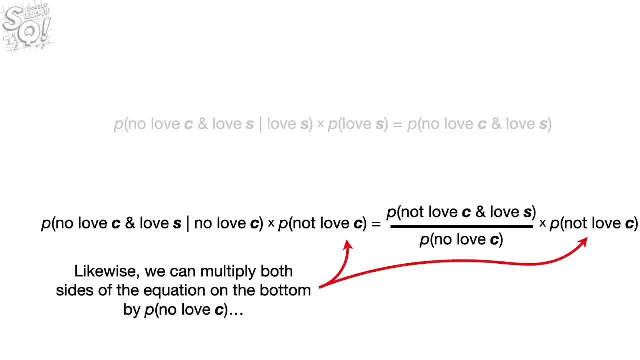 know the probability that someone does not love candy but loves soda, we can still solve for the We ingredients will also get 100% cheaper from the start. Likewise, we can multiply both sides of the equation on the bottom by the probability of not loving candy, And these two terms will be used to square the probability that someone does not love candy. And we are left with the probability that we meet someone that does not love candy but loves soda equal to this stuff on the left side. Likewise, we can multiply both sides of the equation on the bottom by the probability of not loving candy, and these two terms will be lost. 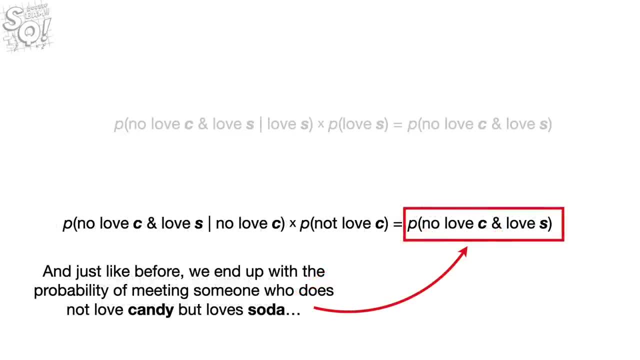 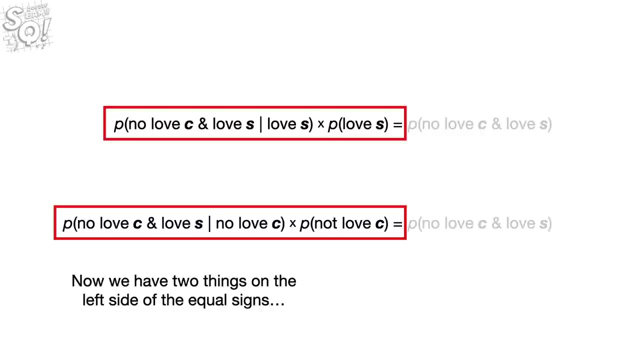 the right side, cancel out And, just like before, we end up with the probability of meeting someone who does not love candy but loves soda equal to this stuff on the left side. Now we have two things on the left side of the equal signs that are both equal to the probability that we will. 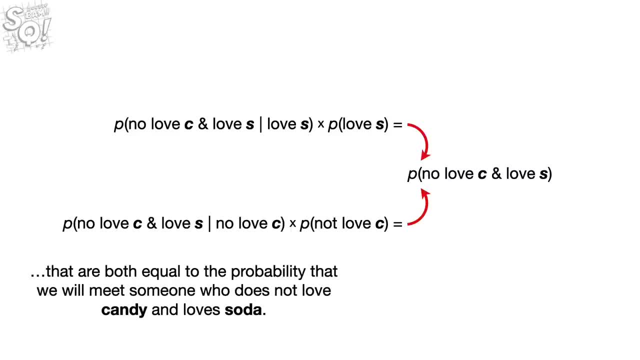 meet someone who does not love candy and loves soda. Now, remember that Statsquatch asked us to solve for this term and this term. without this term, And because both equations are equal to the term we want to omit, both equations are equal to each other, So let's move this up a little. 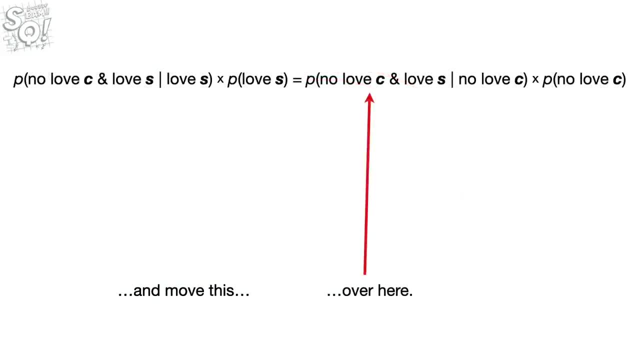 bit and move this over here. Now, remember, we want to solve for this term and we want to solve for this term. We'll start with the term on the left First. we divide both sides by the probability that someone loves soda and the probability that. 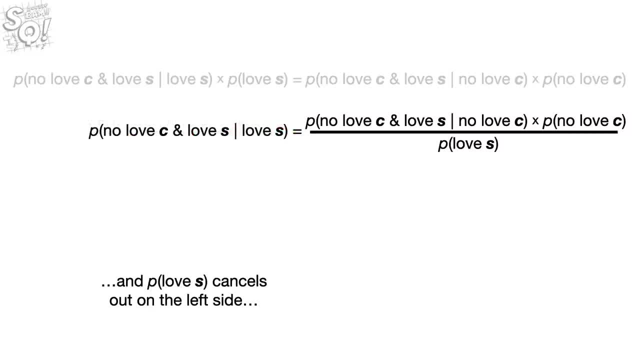 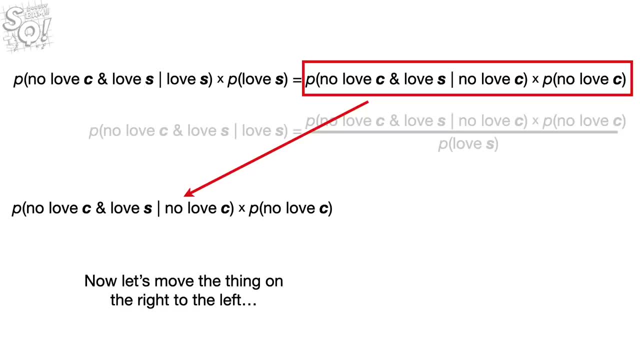 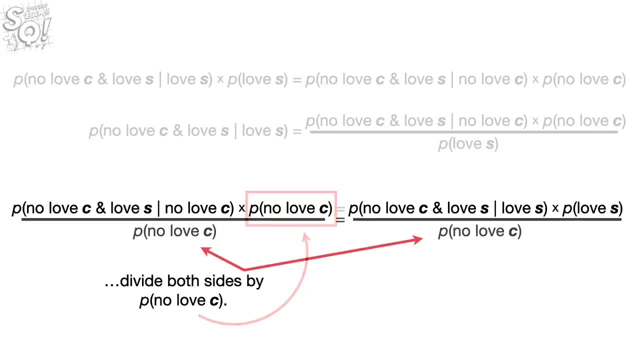 someone loves soda cancels out on the left side. and we have solved for this term Bam. Now let's move the thing on the right to the left and the thing on the left to the right and divide both sides by the probability that someone does not love candy and the probability 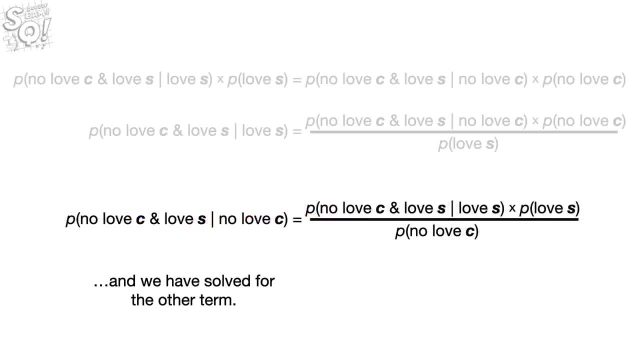 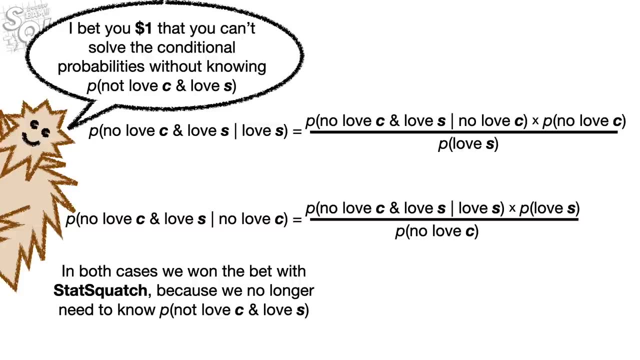 that someone loves soda cancels out on the left side, and we have solved for the other term, Bam. In both cases we won the bet with Statsquatch because we no longer need to know the probability that someone does not love candy and loves soda. But, more importantly, 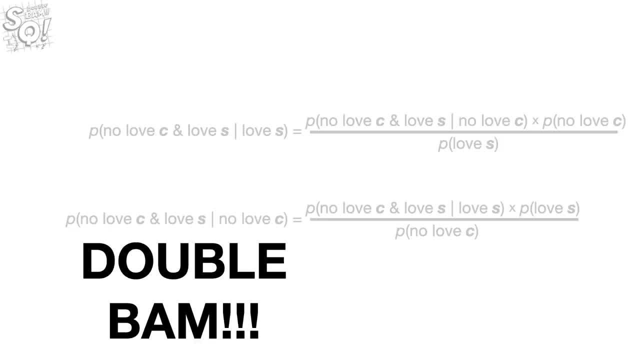 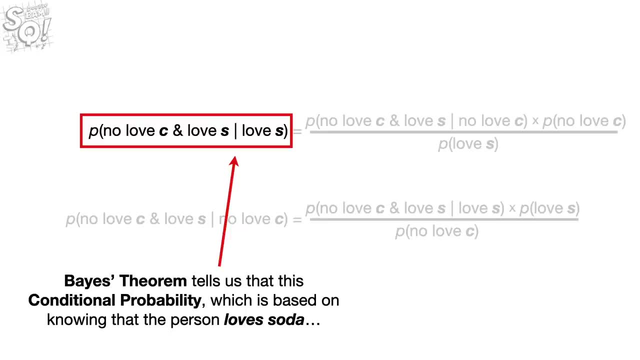 we have derived Bayes' theorem. Double bam. Bayes' theorem tells us that this conditional probability, which is based on knowing that the person loves soda, can be derived from this conditional probability which is based on knowing that they do not love candy. Alternatively, Bayes' theorem. 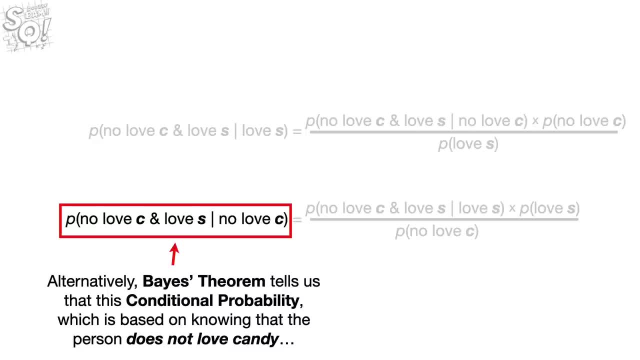 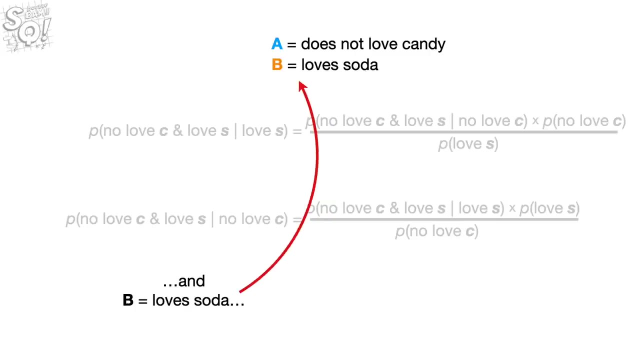 tells us that this conditional probability, which is based on knowing that the person does not love candy, can be derived from this conditional probability based on knowing they love soda In general. if we let A equal does not love candy and B equals love soda, then we can rewrite each equation into the standard formula for Bayes'. 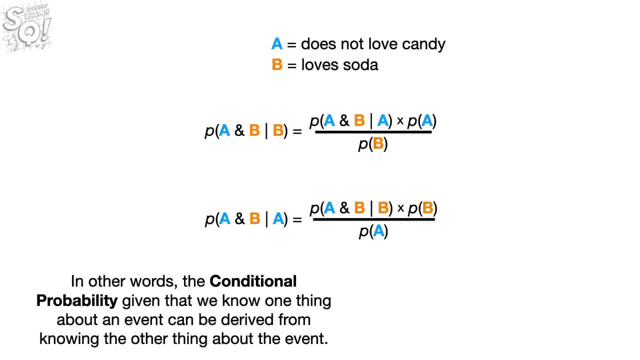 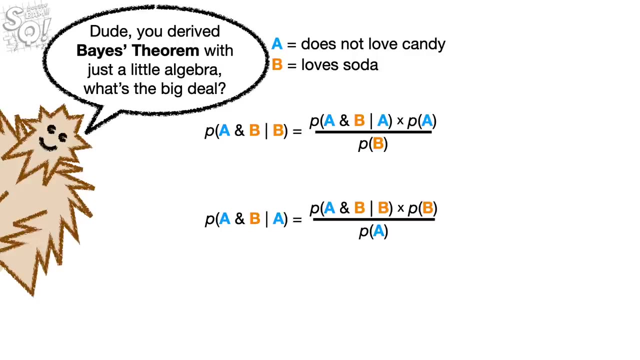 theorem, In other words the conditional probability, given that we know one thing about an event, can be derived from knowing the other thing about the event. Now Statsquatch says: dude, you derived Bayes' theorem with just a little algebra. what's the big deal When we have 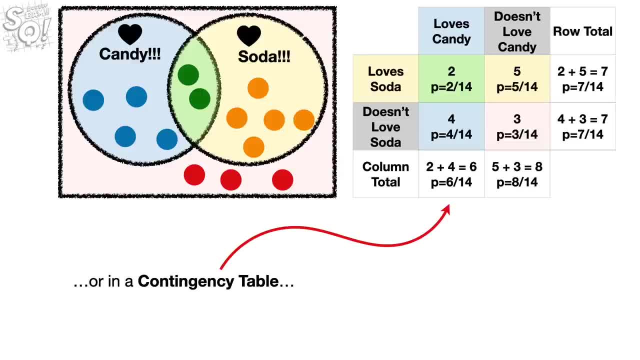 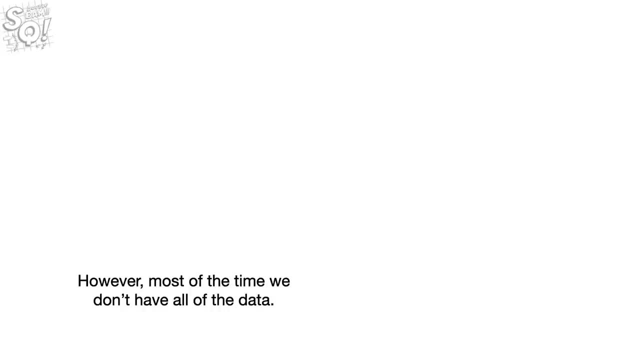 all the data laid out in a nice colorful chart or in a contingency table, then Bayes' theorem is not that big of a deal. In fact, when you have all of the data, Bayes' theorem isn't even a small deal. However, most of the time we don't have all of the data. In other words, 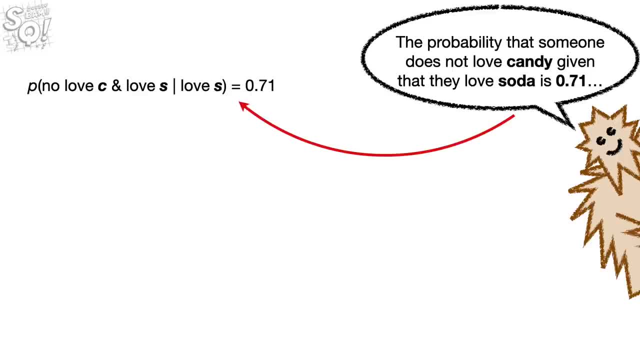 Statsquatch might only tell us the probability that someone does not love candy, given that they love soda, is 0.71, and I'm not certain, but I think the probability that someone loves soda is close to 0.6,. 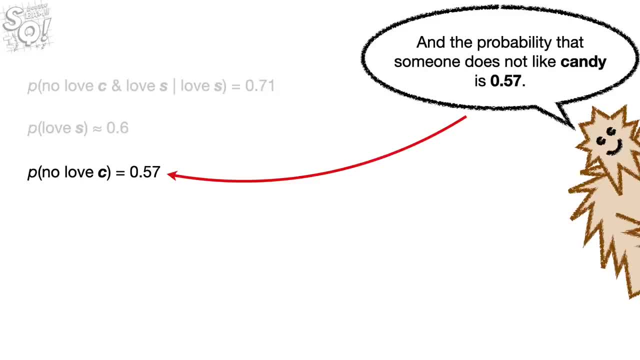 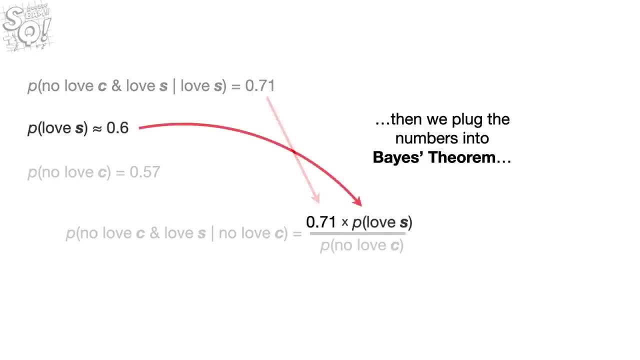 and the probability that someone does not like candy is 0.57.. And if this is all the data we have, then we plug the numbers into Bayes' theorem and get approximately 0.75.. And that means, given this data, which includes a guess about the 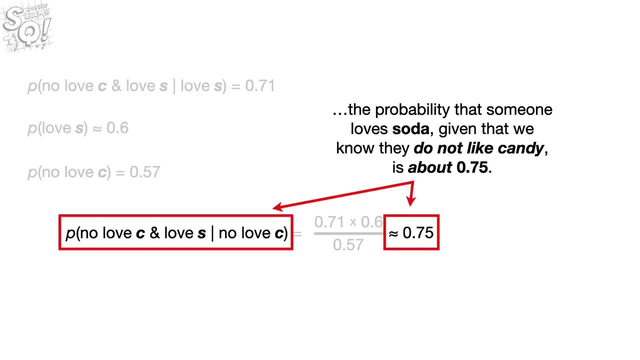 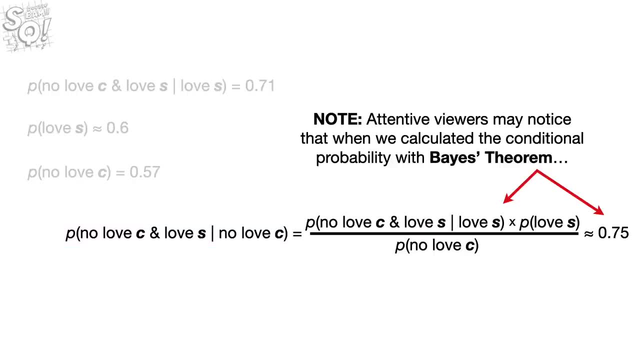 probability someone loves soda. the probability that someone loves soda, given that we know they do not like candy, is about 0.75.. Note: attentive viewers may notice that when we calculated the conditional probability with Bayes' theorem, which we used because we did not have all of 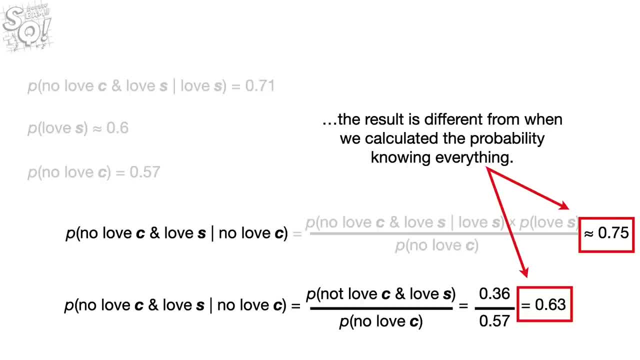 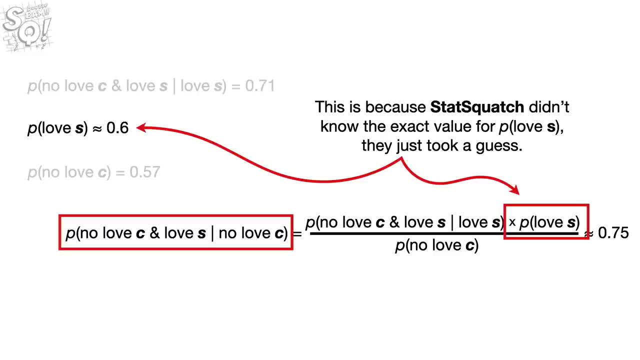 the information. the result is different from when we calculated the probability knowing everything, didn't know the exact value for the probability that someone loves soda. They just took a guess. And while taking a guess might sound like a terrible thing to do, it's the only option. when we have a large population, For example, it would 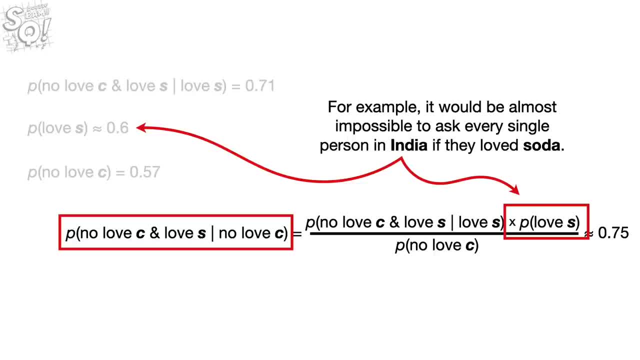 be almost impossible to ask every single person in India if they love soda, So a lot of times we have to make a guess. Bayesian statistics is about understanding what it means to make a guess like this and all it implies. Bayes theorem is the basis for Bayesian statistics, which is this equation paired: 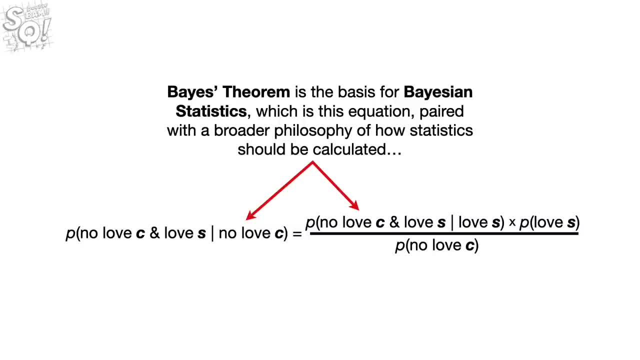 with a broader philosophy of how statistics should be calculated, And we'll cover all these topics in follow-up stat quests. However, before we go, I want to review the standard notation. so if you research Bayes' theorem or Bayesian statistics on your own, you 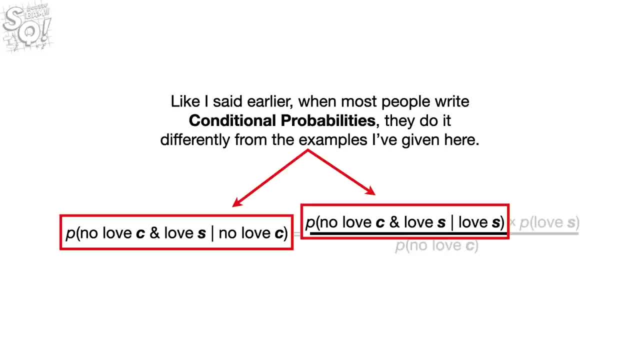 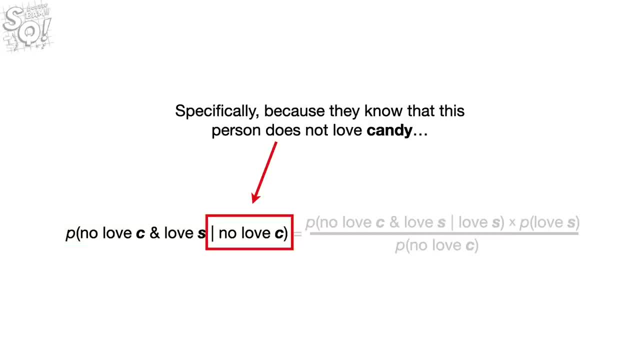 won't be totally lost. Like I said earlier, when most people write conditional probabilities, they do it differently from the examples I've given here. Specifically because they know that this person does not love candy, they do not include it when stating the probability. Now the conditional. 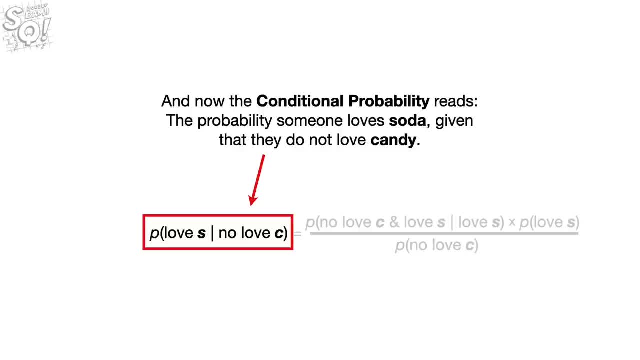 probability reads the probability someone loves soda, given that they do not love candy. Likewise, because they know this person loves soda, they do not include it when stating the probability. Now the conditional probability reads the probability that someone does not love candy, given that they love soda. In the end, it looks like we want to calculate. 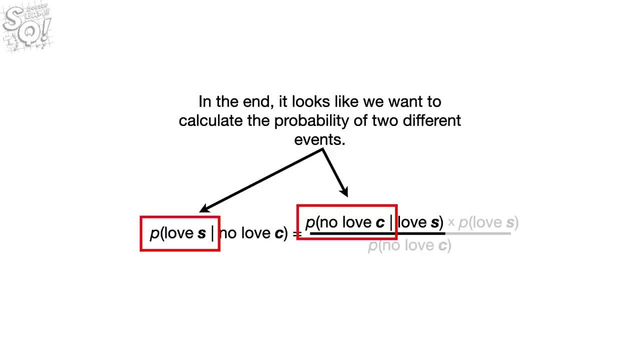 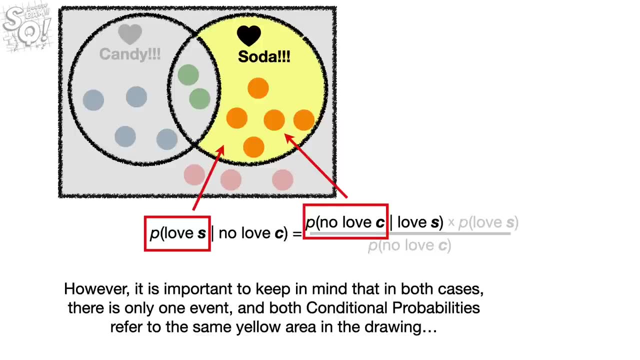 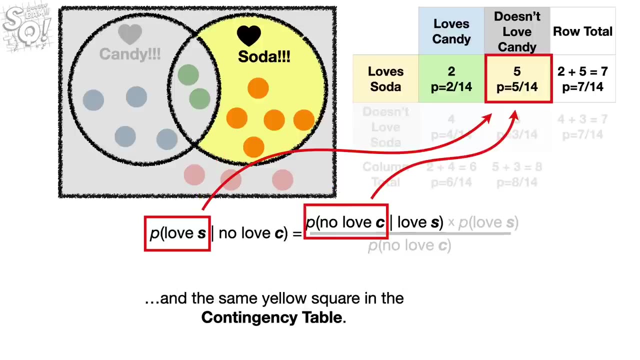 the probability of two different events. However, it is important to keep in mind that in both cases, there is only one event and both conditional probabilities refer to the same yellow area in the drawing and the same yellow square in the contingency table, And the only real difference. 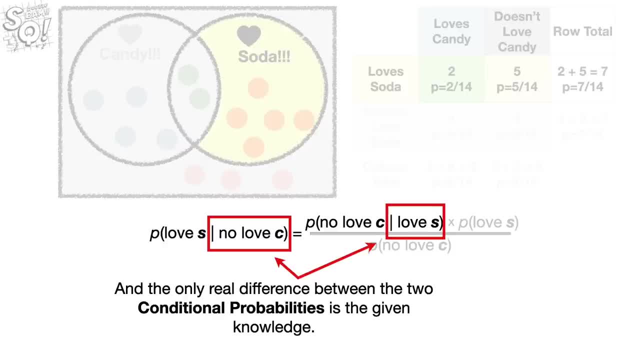 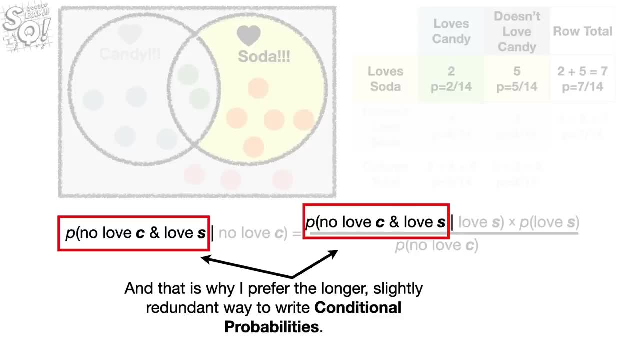 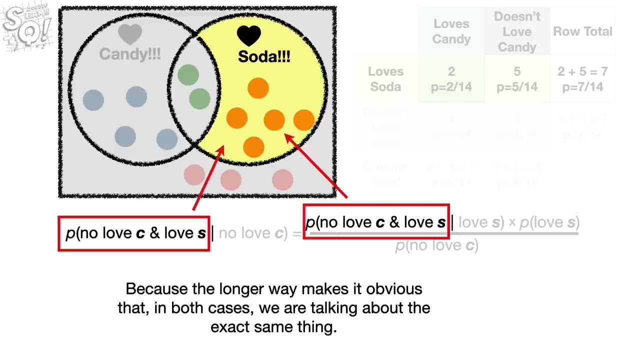 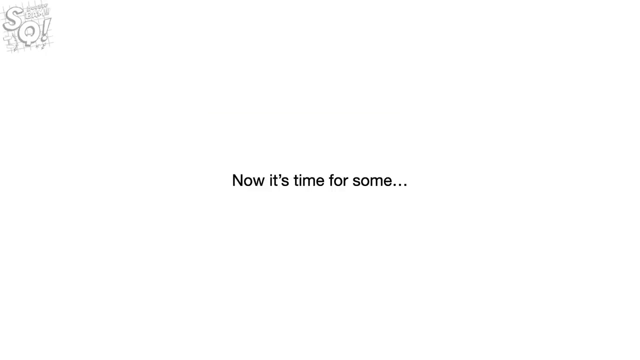 between the two conditional probabilities is the given knowledge, And that's why I prefer the longer, slightly redundant way to write conditional probabilities, Because the longer way makes it obvious that in both cases we are talking about the exact same thing. Now it's time for some shameless self-promotion. If you want to review statistics and machine 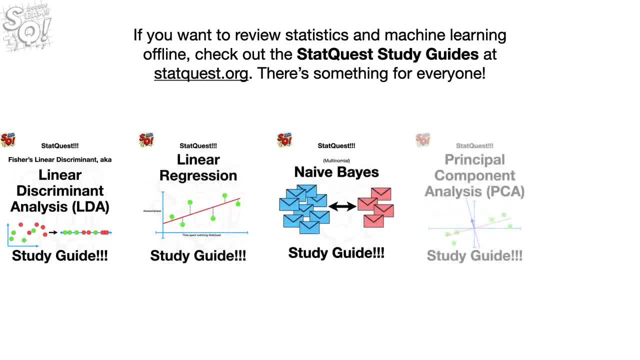 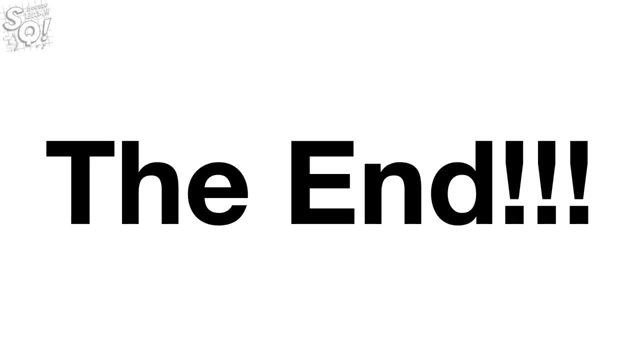 learning offline. check out the StatQuest study guides at StatQuestorg. There's something for everyone. Hooray, We've made it to the end of another exciting StatQuest. If you like this StatQuest and want to see more, please subscribe. 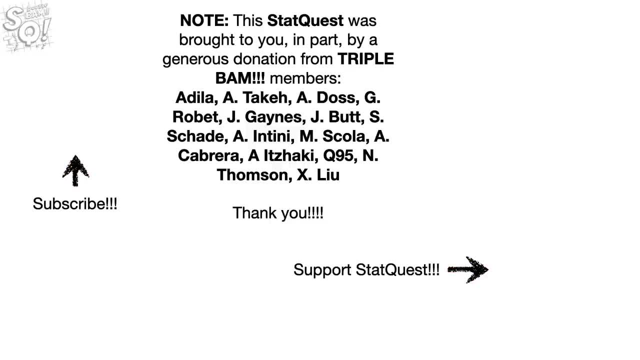 And if you want to support StatQuest, consider contributing to my Patreon campaign, becoming a channel member, buying one or two of my original songs, or a t-shirt or a hoodie, or just donate. The links are in the description below. Alright, until next time. quest on.